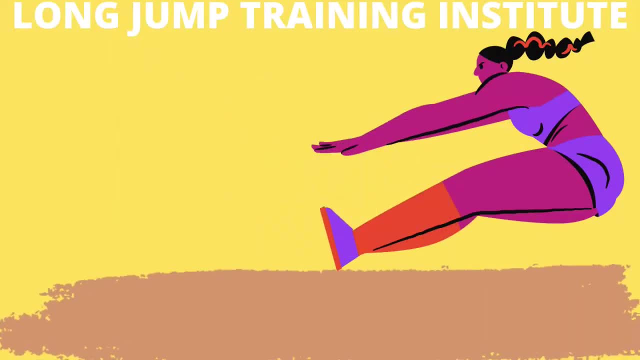 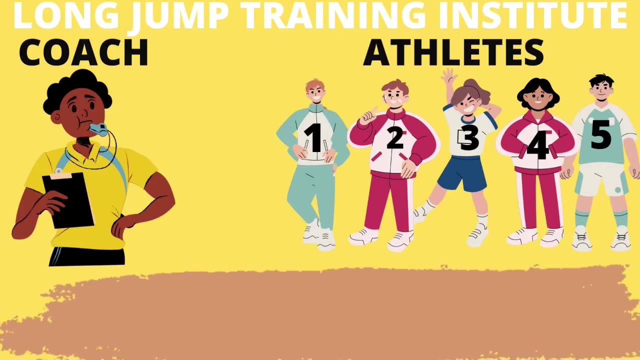 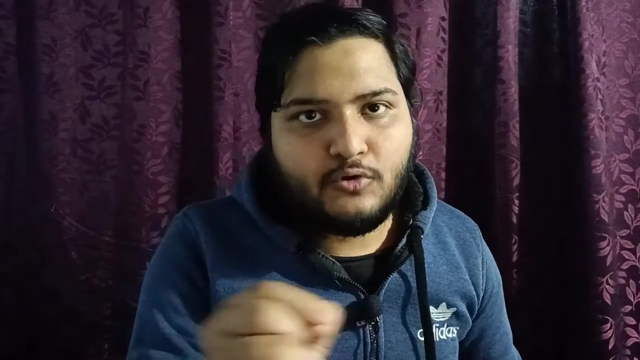 there's a training institute for all the long-term athletes. so in this institute a coach has been training all the athletes into the institute for a duration of one month and the committee after the one month they'll be deciding upon whether we should keep this particular coach or not. so, friends, 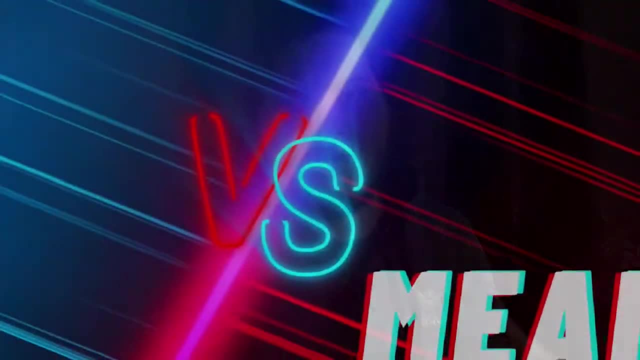 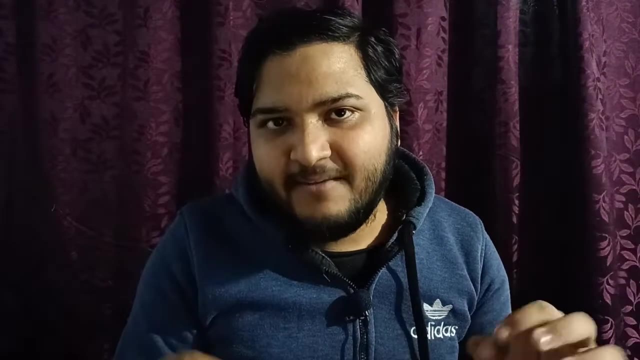 let us understand this problem using the mean and and the median function. so, using the mean and the median function, the committee will be deciding upon whether the at least performance have been improved or not, or they have been depleted day by day. so friends will be using this example to 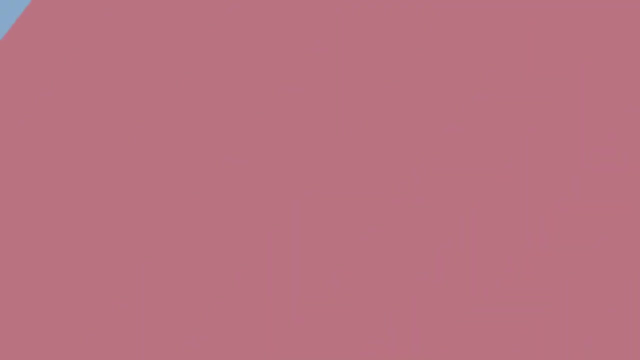 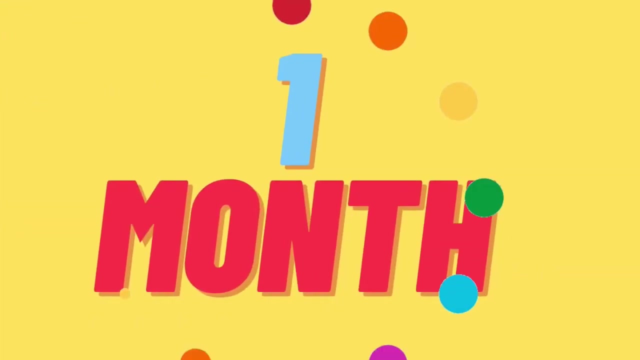 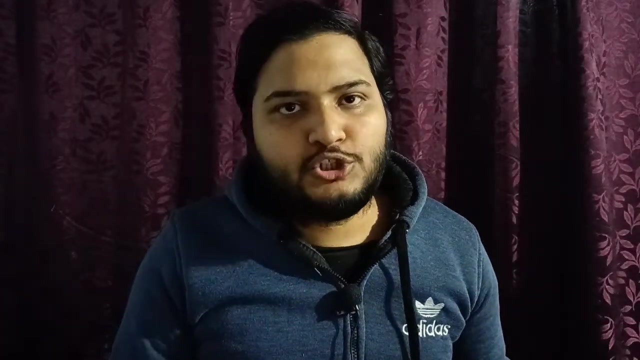 determine whether the athlete should be preferred over the mean value. let's move to our example. so let us suppose that there are five different athletes into the coaching institute, so, and the one month training has been completely the improvement produced by the five different athletes with the help of the coach. so the very first player has improved his performance by 0.15. 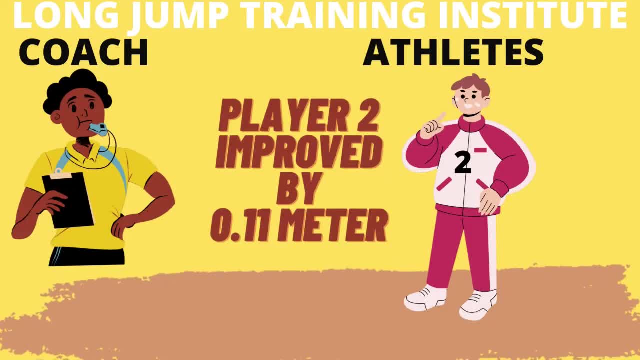 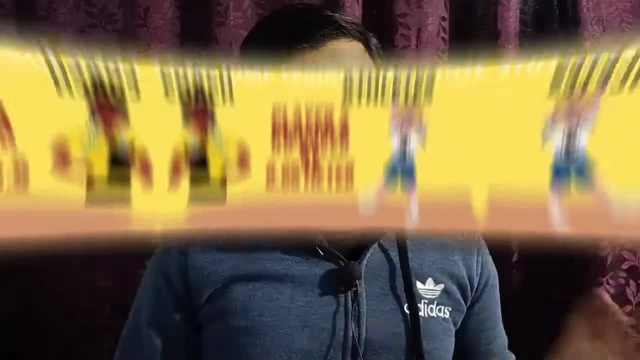 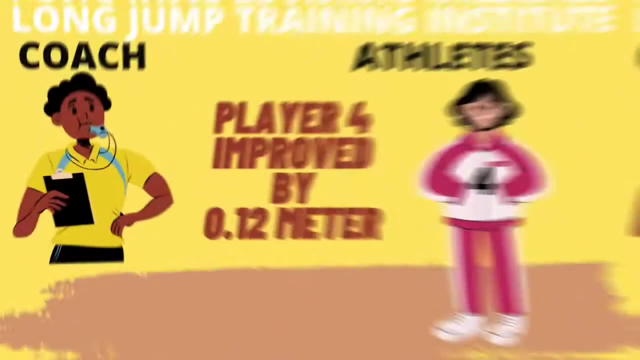 meter. the second player: he has improved his performance by 0.15 meter. one meter. similarly, the third player: she has improved her performance by 0.06 meter. and the fourth athlete: she has improved her performance by 0.12 meter. now the last athlete, he has degraded. 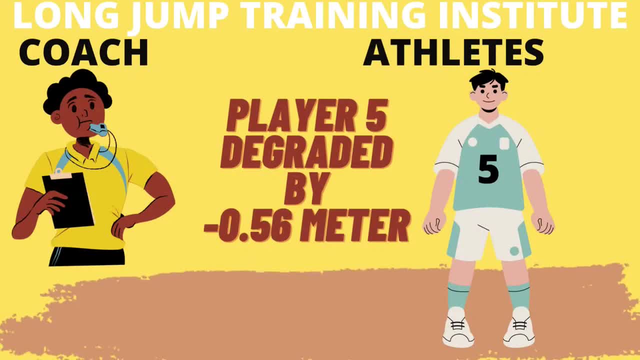 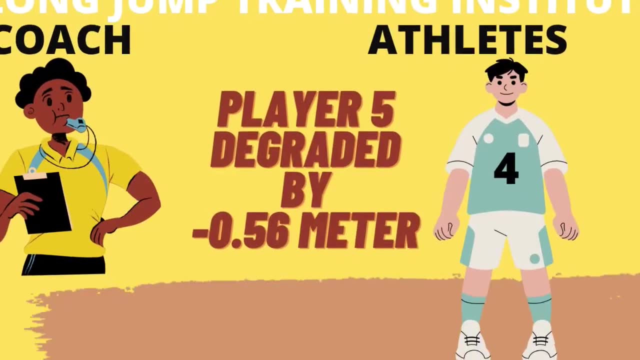 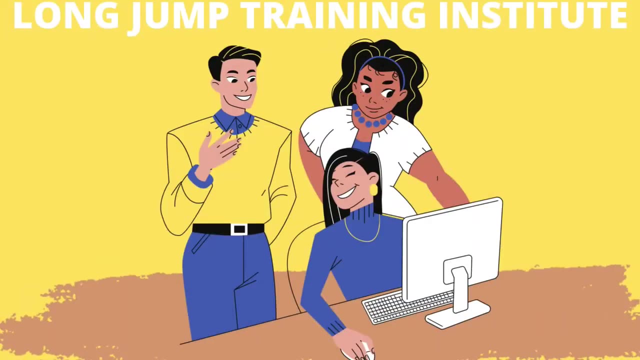 in his performance and he is now jumping less than what he was doing earlier before the coach. so, friends, he is jumping less by minus 0.56 meter now. the one month duration has passed away. now let us see what the committee will decide or not, whether the coach should be kept or not. 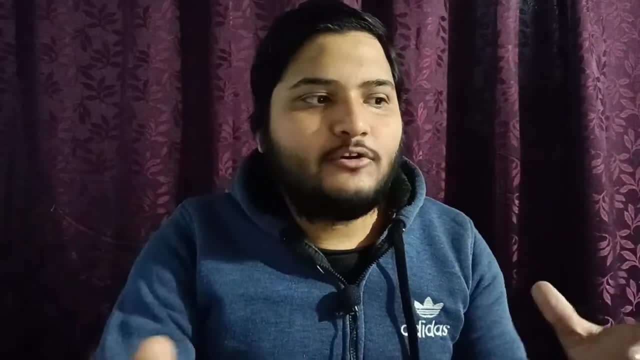 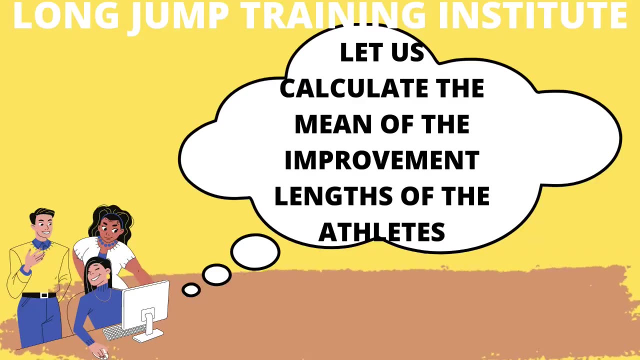 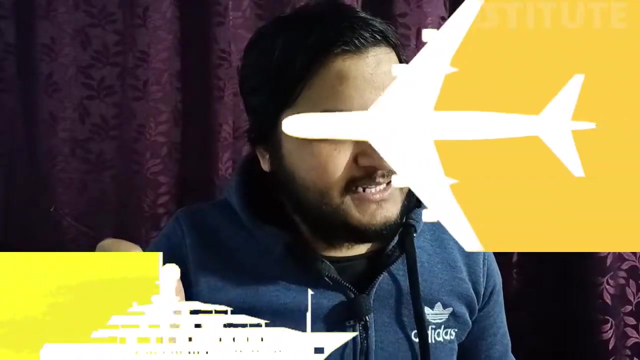 into the institute. so committee thinks on calculating the mean value of the improvement produced by all the five different athletes. so they noted down all the improvement points. so the very first athlete, he improved by 0.15 meter. the second athlete, he improved by 0.11 meter. the third athlete, by 0.06. 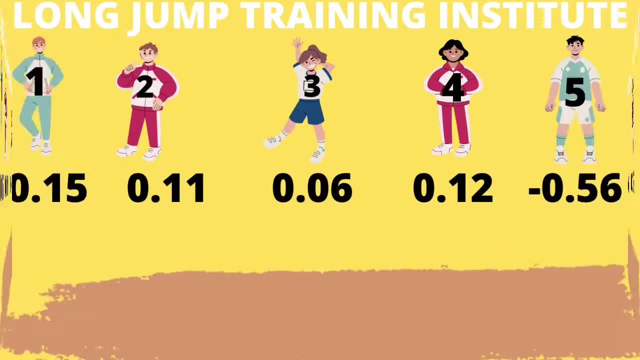 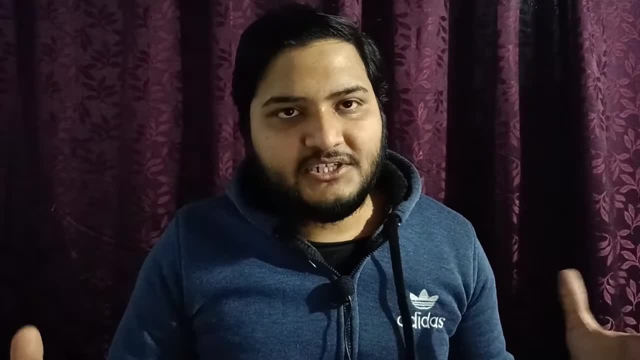 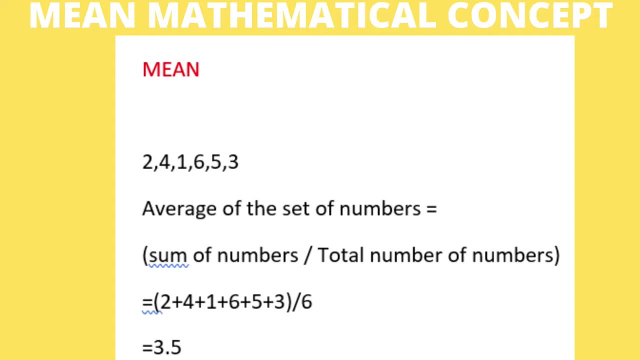 the fourth one by 0.12, while the fifth one degraded himself by minus 0.56 value. now for calculating the mean function. you have this particular formula onto the screen, so you can just pause a while and then look into this. how do we calculate the mean value from a given set of? 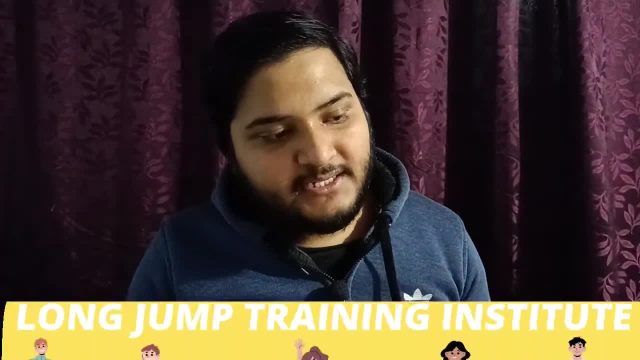 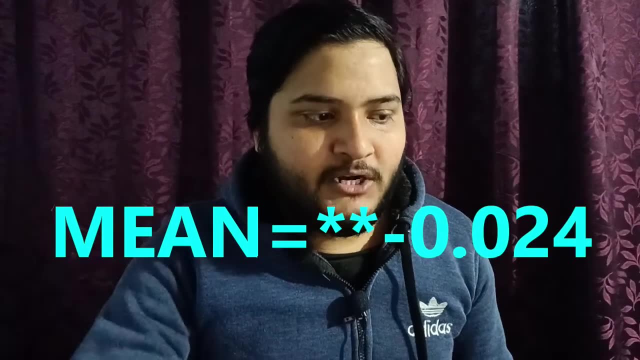 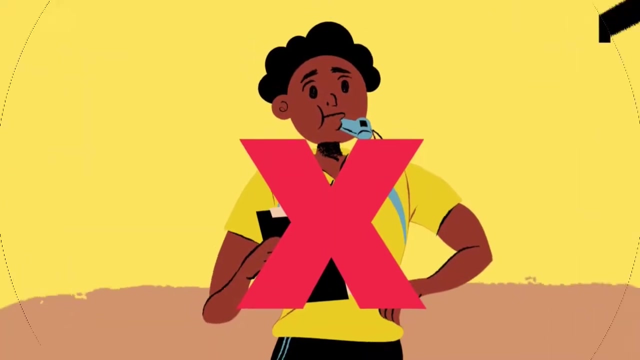 numbers. now the committee sat down and they calculated the mean value using that particular formula. you can see the mean value was minus 0.12 meter. now what does this show? this shows that the coach has failed into his duty. he has completely ruined all the athletes. he has degraded all the 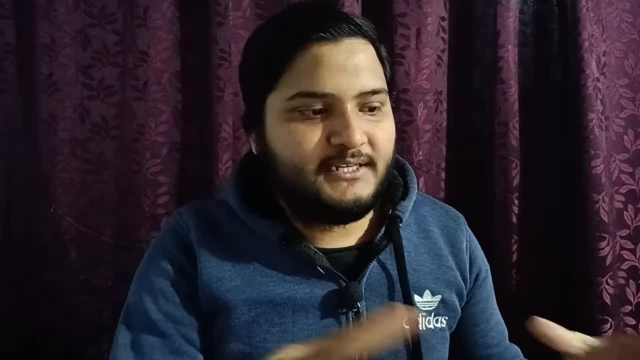 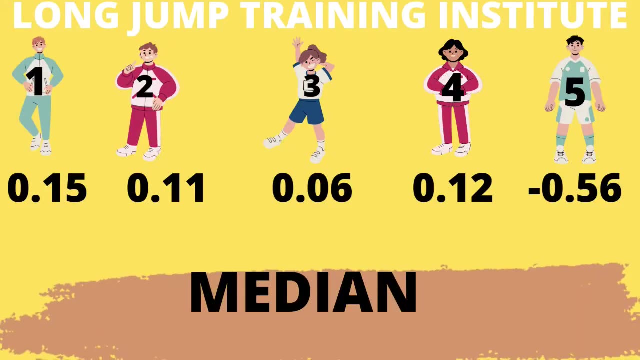 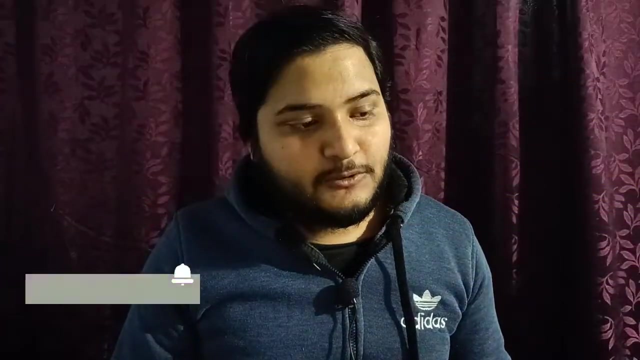 athletes performance in the time which he was doing his duty. but is it like that? let us quickly see using the median function. see the median function. so these are all the improvement numbers which are produced by all the athletes into the coaching institute. now to calculate the median, first of all we need to 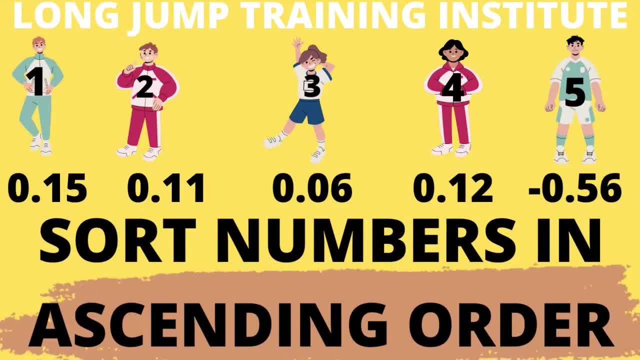 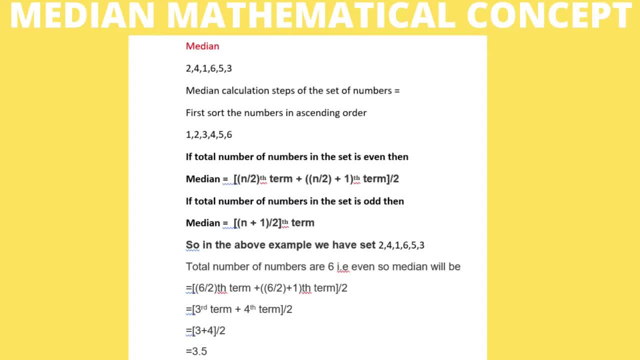 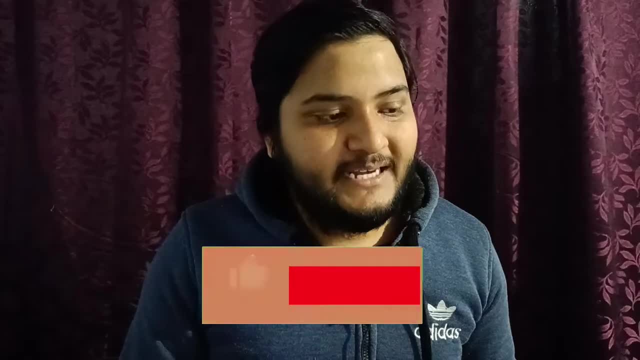 sort the numbers in the ascending order for more information on how do we calculate the medium value you can see onto the screen we have. i have provided all the steps through which and and an example through which you can clearly understand how do we calculate the median value. 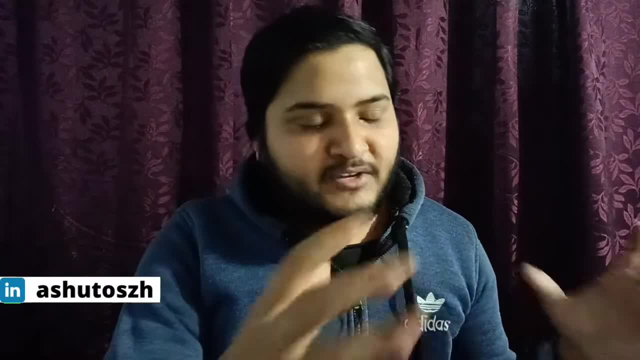 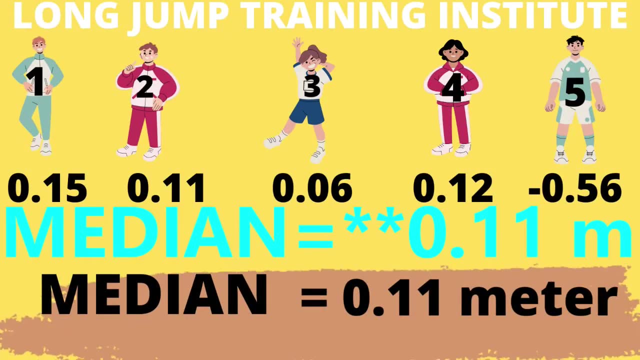 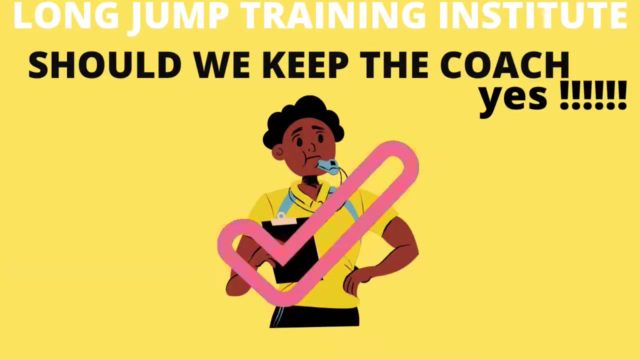 so, friends, now the median of this particular function. after doing a lot of analysis and using that particular function, we get 0.12 meter. now you will think that the median is the correct value and that is providing the right insight on whether we should keep the coach or not. 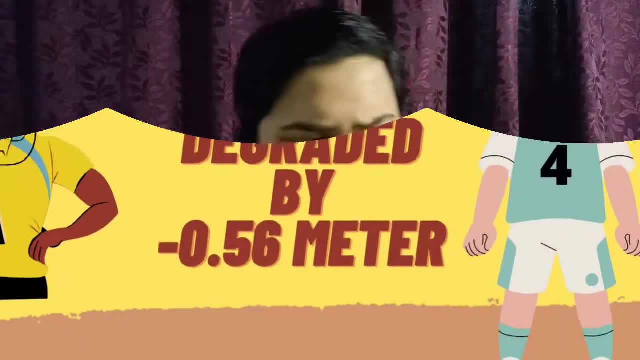 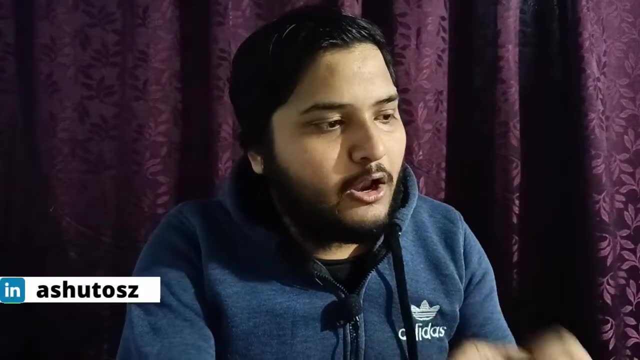 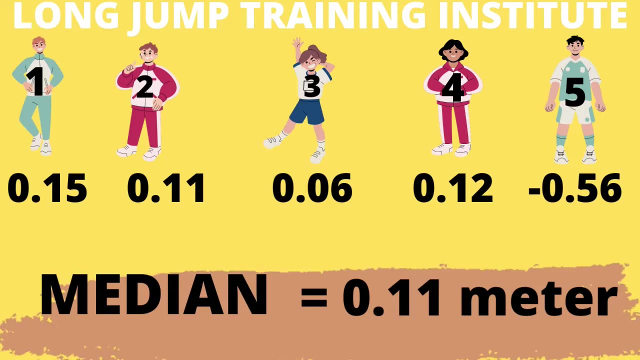 and the answer is we should definitely keep the coach. if you look at the numbers, how the minus 0.56 value is providing or degrading a lot our analysis, so it is. it is completely ruining our analysis and it is not providing a good result to us, while if 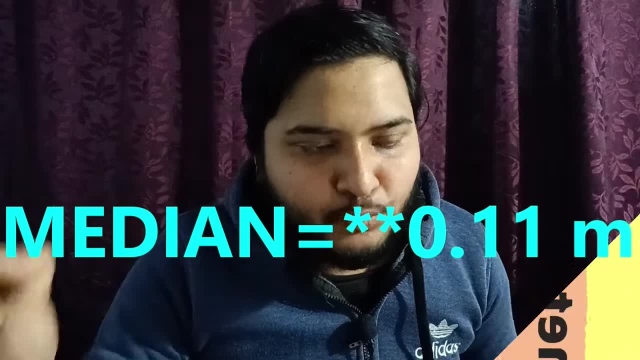 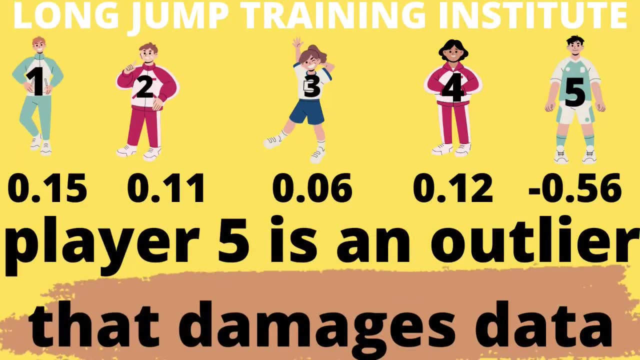 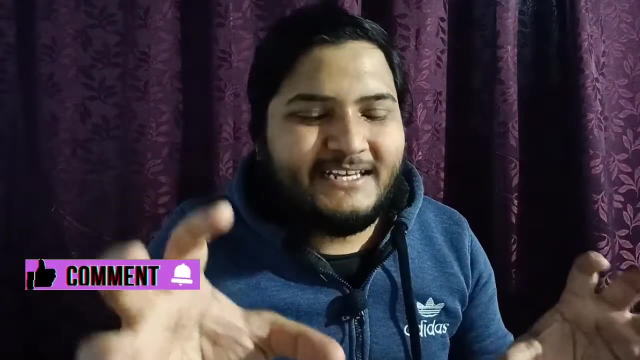 we use the median function, it is giving us 0.12 meter value and that is the correct value and the coach should be kept in that particular institute. now, minus 0.56 value in this particular set of numbers of five different set of numbers that is depleting or ruining our results. that is, that number in a particular data set is called as.